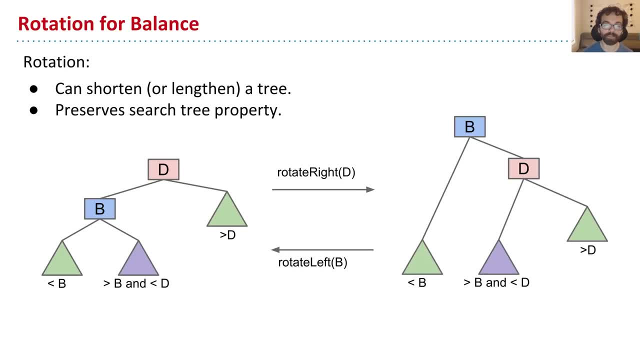 effect on the height of the tree And, very importantly, it preserves the search tree property. So here is just an alternate cartoon hammering home what exactly rotation is Here: D is the root and as a left child, which is B, And then these triangles represent subtrees of. 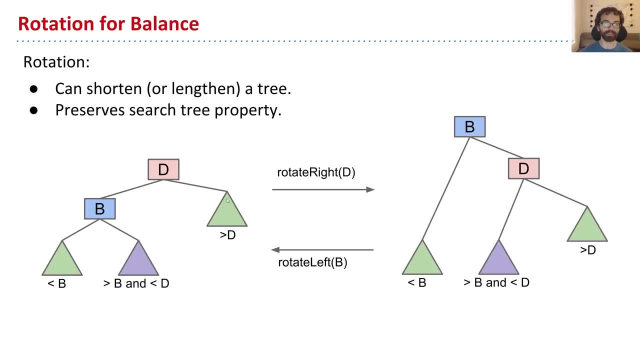 the items that are less than B, between B and D, and then these triangles represent subtrees of the items that are less than B, between B and D and greater than D respectively. Now, when we do the rotate right operation, we see that D goes down into the right and B its former left child. 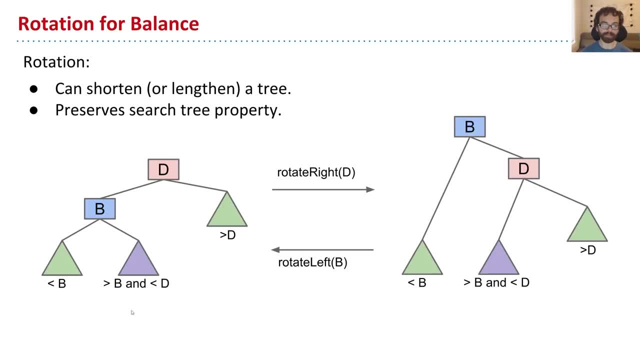 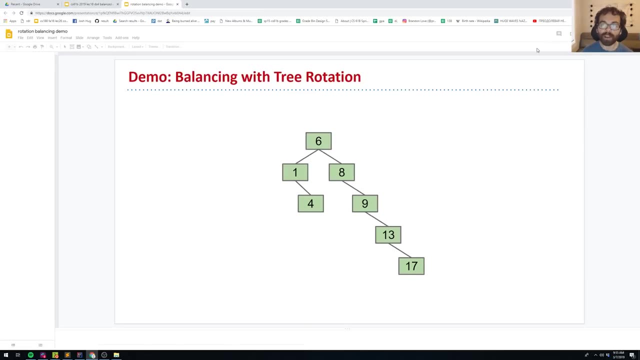 is the new boss, And naturally the items that were between are transferred from being B's subordinates to D's subordinates, And so we can use this process in general to balance a tree. So let me show you a bigger example than the tiny one you did, just to drive home that this is really 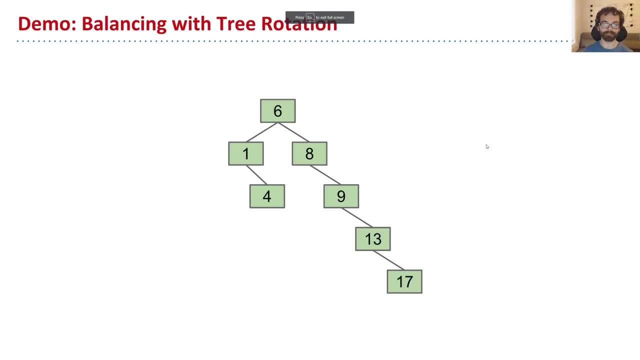 truly possible. You can take trees and balance them using rotation. So here is a tree that is not balanced. It's not so great, but it has one, two, three, four, five, six, seven items. Now, if you think, what is the bushiest tree that I could possibly get? I should ultimately be able to get a. 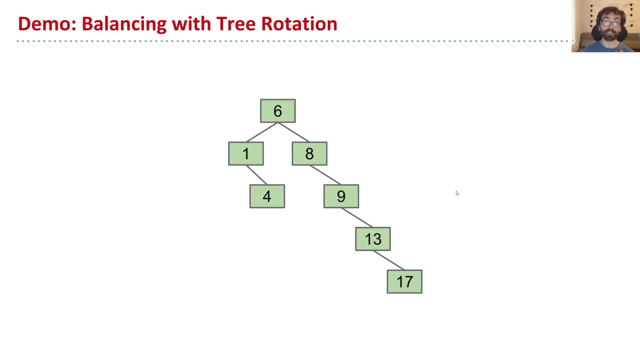 tree that is only height two instead of four. So to do this, I'm going to perform a sequence of rotation operations that seem intuitively correct to me, but it would be hard for you to probably balance this on your own, So I'm going to pick arbitrarily. it seems that I want to rotate nine to the left, And you'll see. 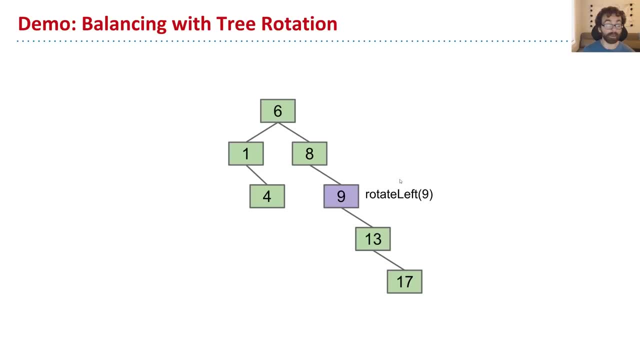 the result of this in a moment why it seems to make sense. So this is a totally arbitrary choice that should not seem natural to you at all. So when I rotate nine to the left- this nine and this 13, they interact. You can think of them as temporarily merging, and then nine gets sent down. 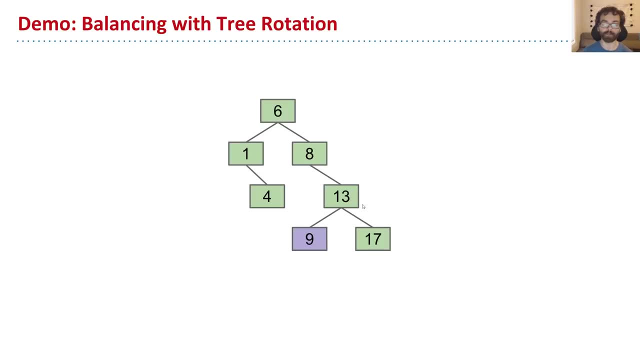 and to the left, And so the end result is: my tree is a little shorter, which is pretty nice. Now, how would I know that the tree is a little shorter? Well, I would know that the tree is a little shorter than the tree itself. So how would I know that the tree is a little shorter than the tree itself? 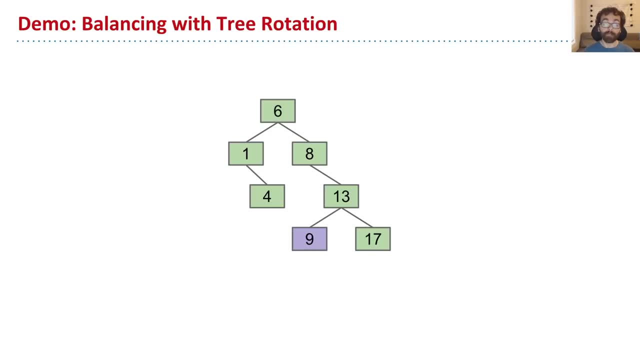 So how would I know that the tree is a little shorter than the tree itself? Well, I just saw it intuitively, And we're going to be describing ways to pick the right tree rotations later in this lecture. OK, so next I might pick that. I want to rotate six to the left. So here the rough. 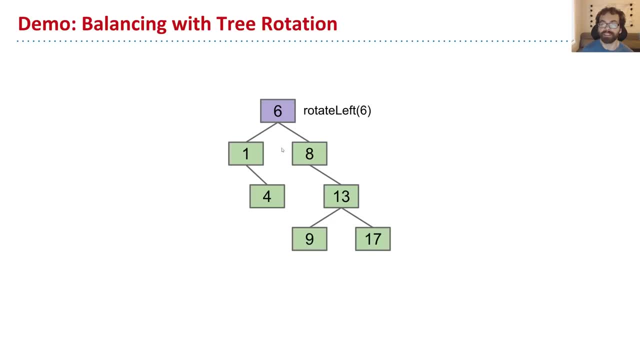 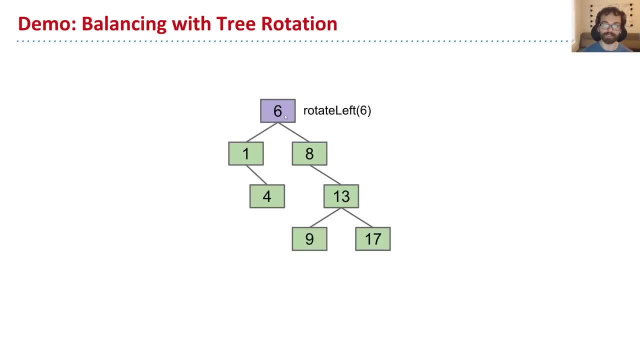 child. So six and eight will be temporarily merged And then six gets down and to the left sent down and to the left to be eight's new left child. So that is the result of the rotation And if that's not totally clear, maybe pause the video and try it yourself and say: 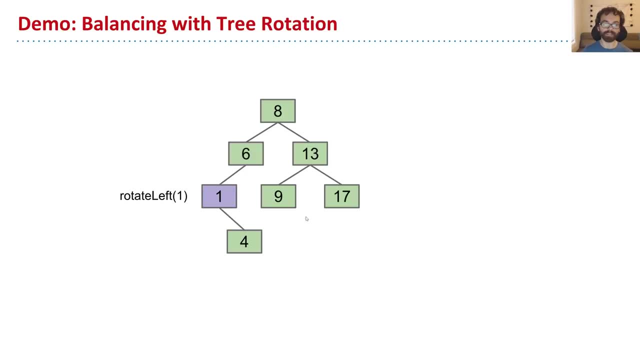 OK, I get it All right. next I might rotate one to the left, And when I do this, one and four will be temporarily merged And one will go down and be sent to the left. Now I should note here: 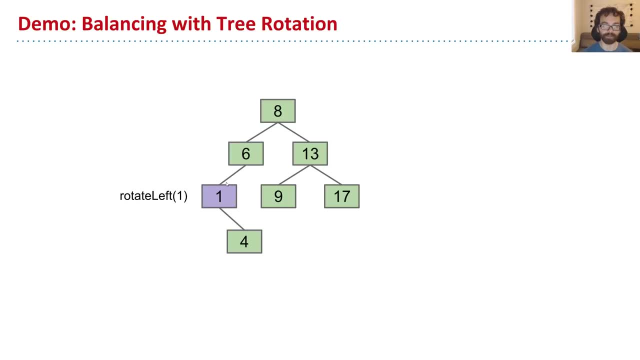 you might ask yourself what would it mean to do rotate right in this circumstance? The answer is: it's undefined. There is no meaning to saying rotate one to the right, because that would mean that we're going to make the left child the new boss, which wouldn't make sense. We can't have a 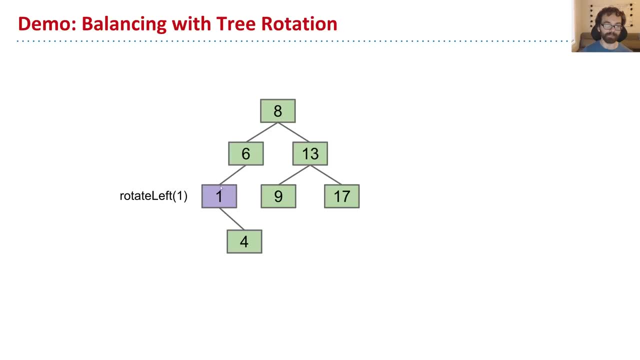 null, sitting in the middle of the tree. So we can only rotate left when an item has only a right child. OK, so anyway, the result of this rotation operation is that one ends up down here. No stop, All right, And so next. 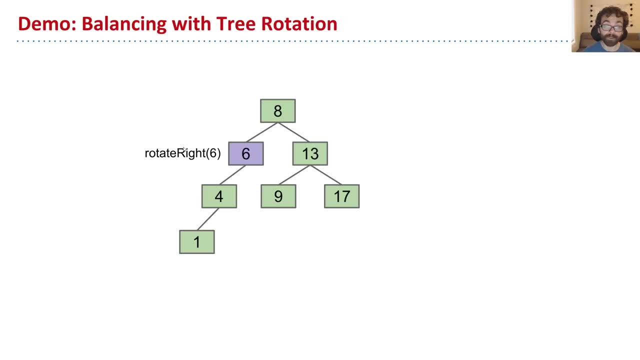 we're going to rotate six to the right And in this case, the reason I'm doing this is, well, it's the last step in my balancing operation And it kind of mirrors just a little bit the problem you had before. So notice, this shape became this straight line shape, And now, if I rotate six to 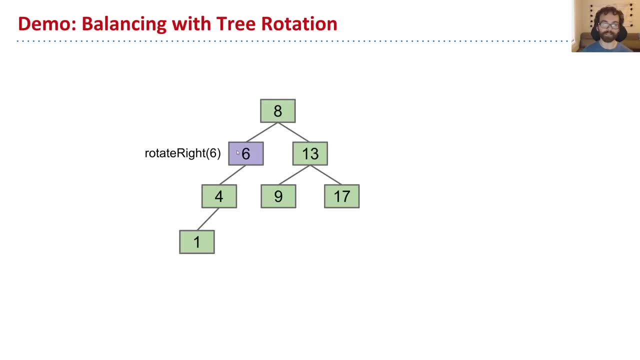 the right. what will happen is four and six will be temporarily merged And six gets sent down into the right, So I don't expect you to be able to see this tree and recognize. these are the rotation operations I need. However, I do think at this point you should understand how each of the rotations worked and how. 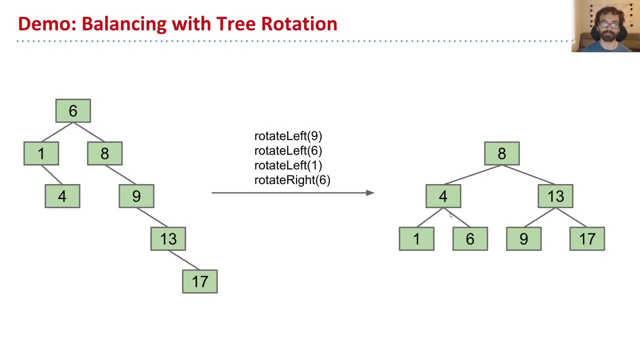 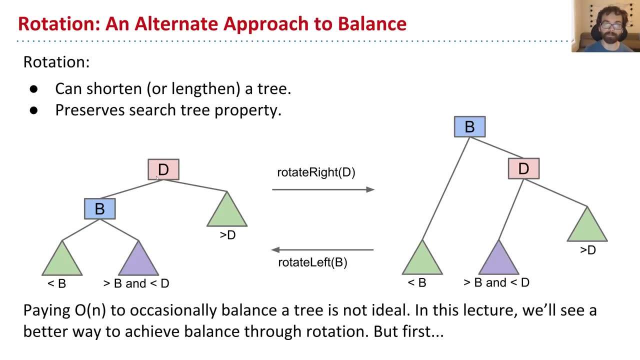 ultimately, we ended up with a nice balanced tree, All right. Now what we don't have at this point is any kind of algorithm for specifically deciding which rotations to do Like. we just saw that it's possible, but we don't have a specific algorithm. So paying. you could, in theory, do this, though.